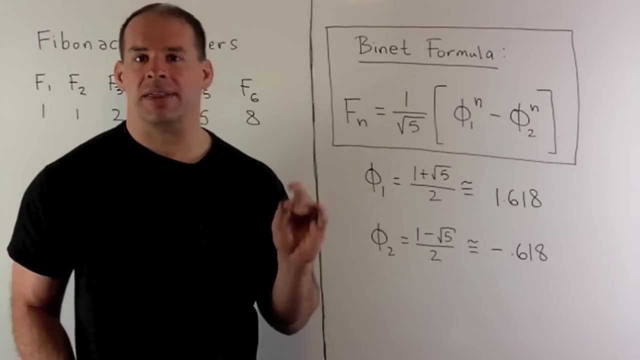 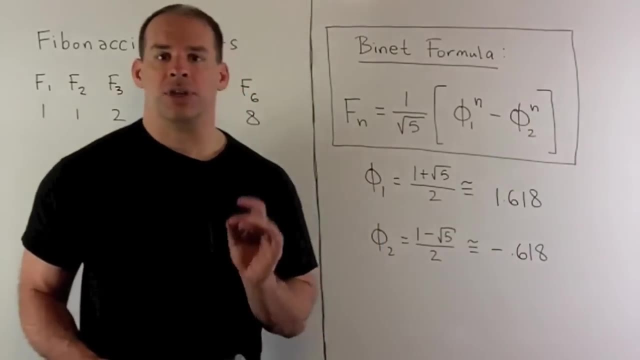 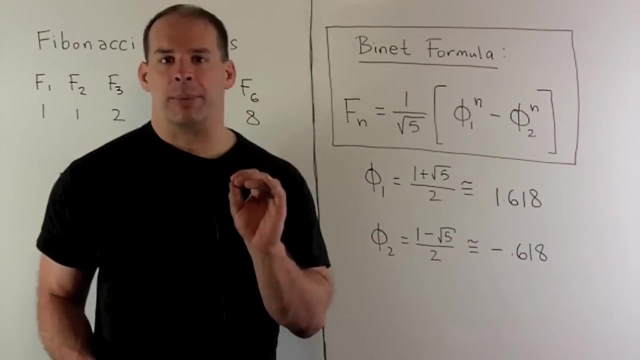 I raise both to the nth power, take the difference and then divide by square root of 5. That gives me the nth Fibonacci number. So that seems pretty unlikely. This is always going to be an integer. So let's take a look at a few examples before we get to the linear algebra. 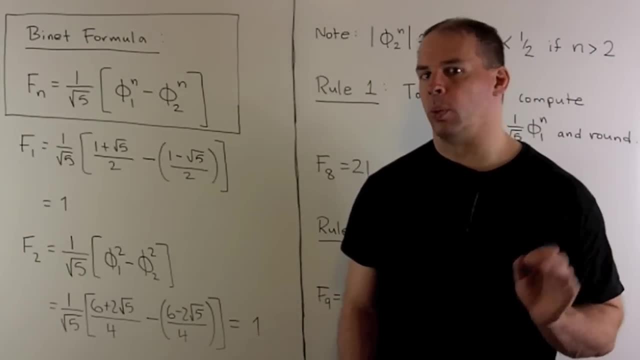 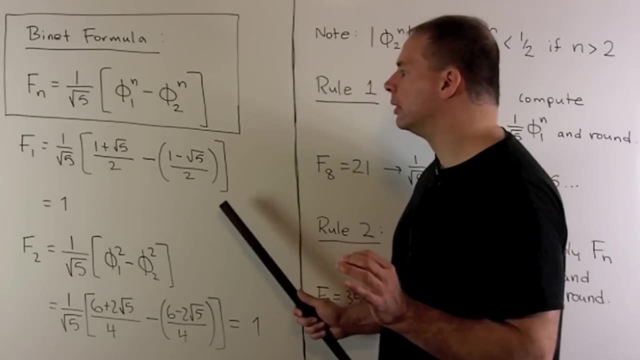 First let's verify that F1 and F2 are equal to 1 using our formula. So if I let n be equal to 1, we get this expression here. The term on the inside is going to collapse to a square root of 5.. 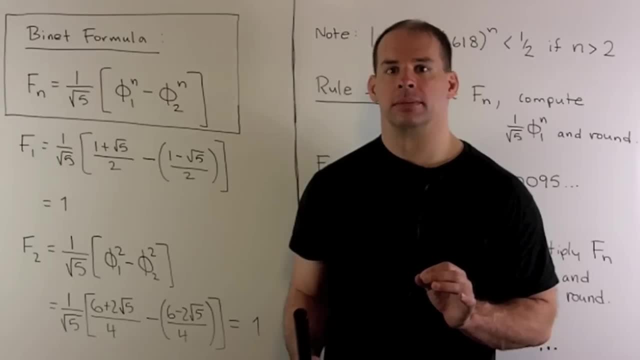 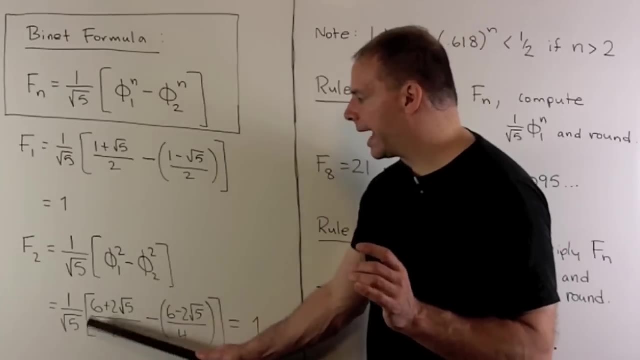 So we get a 1 to come out and that checks. Then, if I let n be equal to 2, we have to work out both of these squares. When I do that, so that's this expression here that collapses to a square root of 5.. 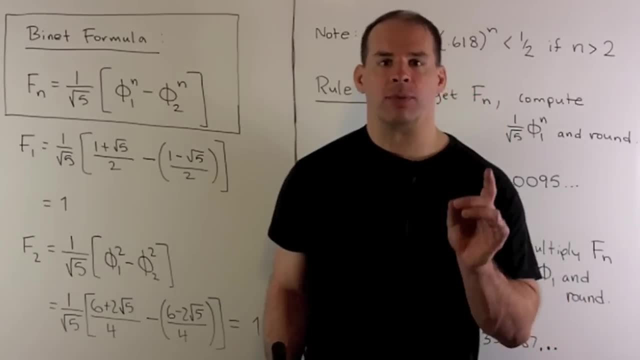 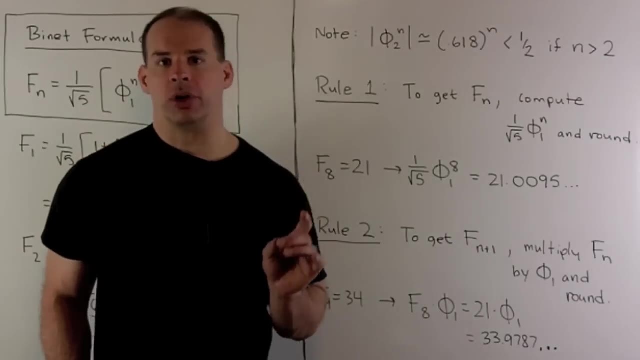 And again a 1.. And again a square root of 5 comes out. So F1,, F2, check Now for the higher numbers. we do a little bit of trickery. So we know for Phi, 2, okay, that's roughly minus 0.618.. 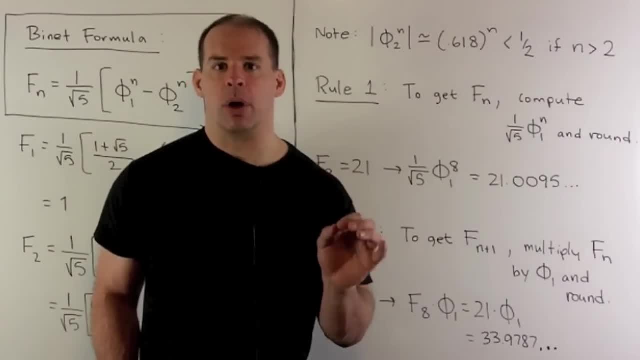 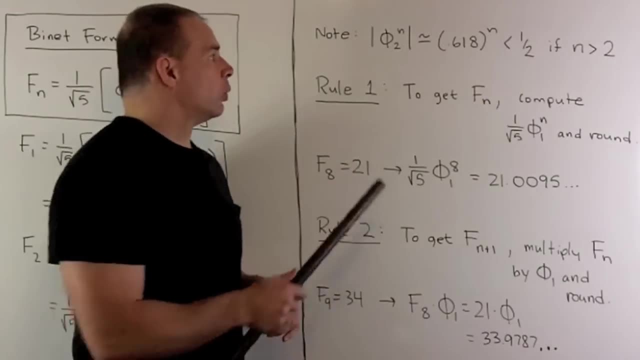 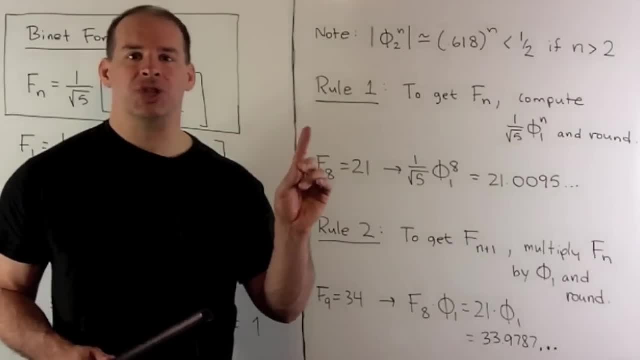 So the idea is going to be: when your n is far out enough- say bigger than 3 or 4, well, we can ignore that term. 1 raised to the nth power and then just round. So let's check that for a specific example. 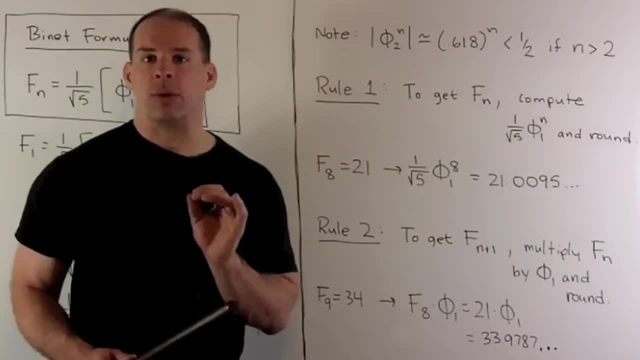 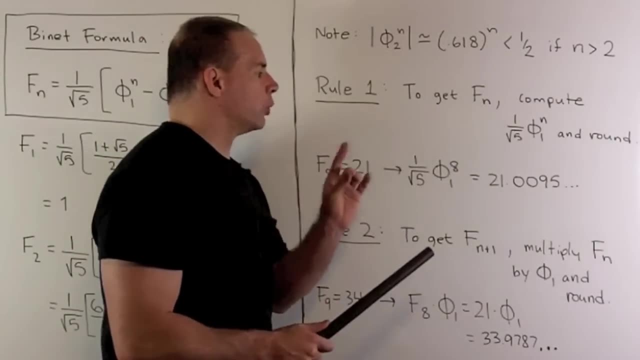 So if I have f sub 8, on the previous board we worked out that that was 21.. I take 1 over square root of 5, multiply by 5, 1 to the 8th power, we're going to get 21.0095, and so on. 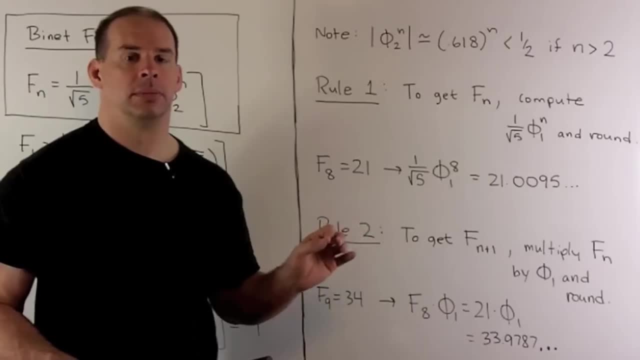 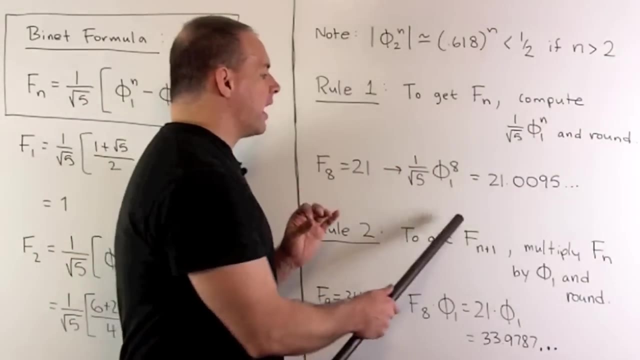 So that comes out pretty close. Another rule we can use again if your n is out a little bit: if I want to get f sub n plus 1 from f sub n, all I need to do is multiply by 5, 1 and round. 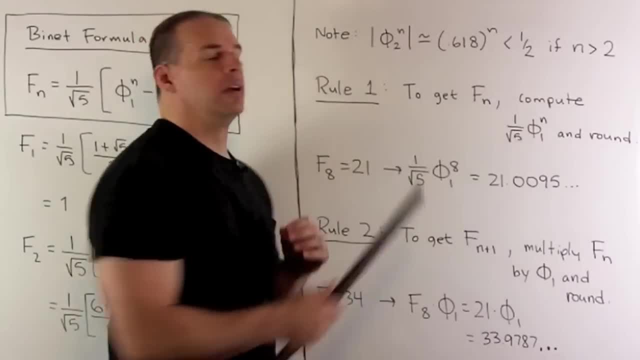 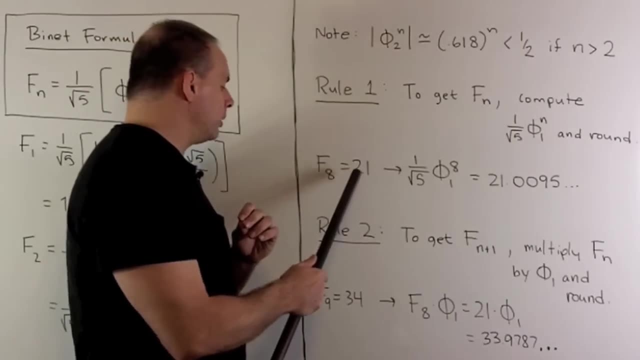 Okay, it's the same idea here. You can ignore the effect of 5: 2.. Now we start with: okay, our f sub 8, equal to 21,. and I want to get f sub 9, equal to 34.. 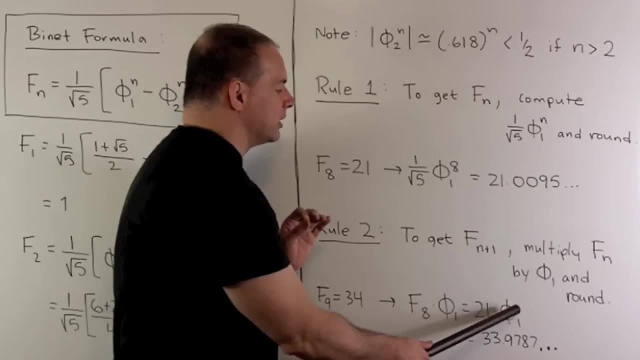 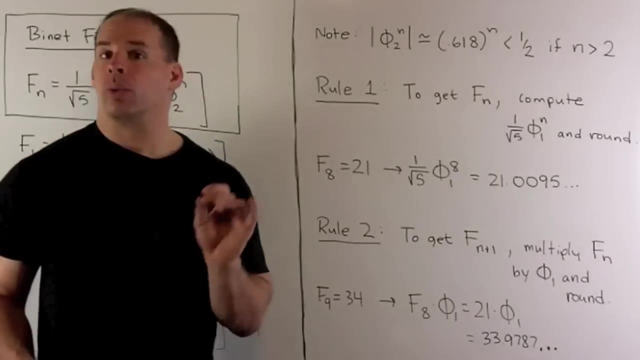 We're going to take f sub 8 times 5: 1. So it's 21 times 5: 1.. Work it out with the calculator. I get 33.9787, and again we're pretty close. Let's bring in the linear algebra. 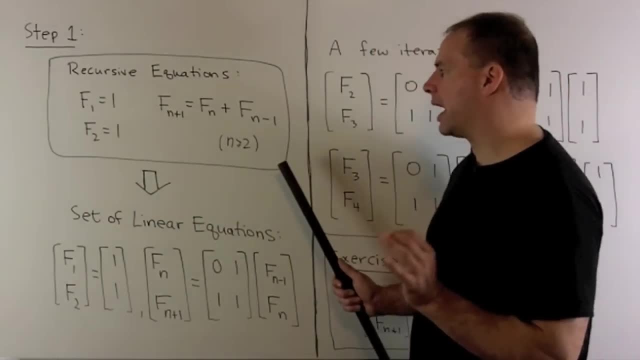 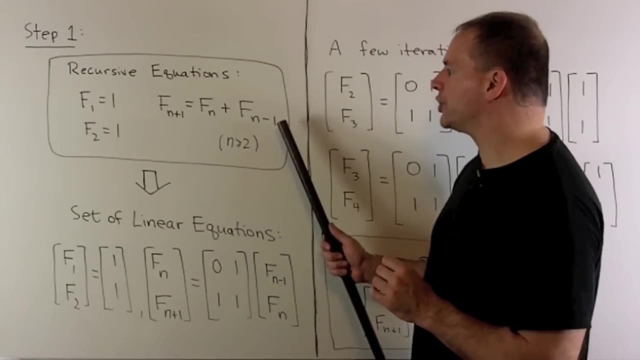 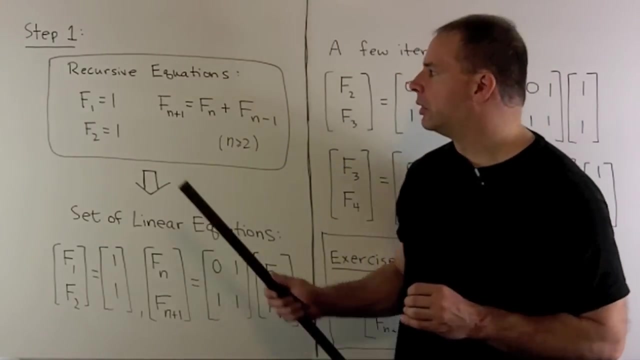 First step we'll take the defining relations for the Fibonacci numbers. We're going to encode them in matrix vector form. So, if you note, here this is a linear equation, So we can set this up as a matrix vector product. Now we have f1 equals 1, f2 equals 1.. 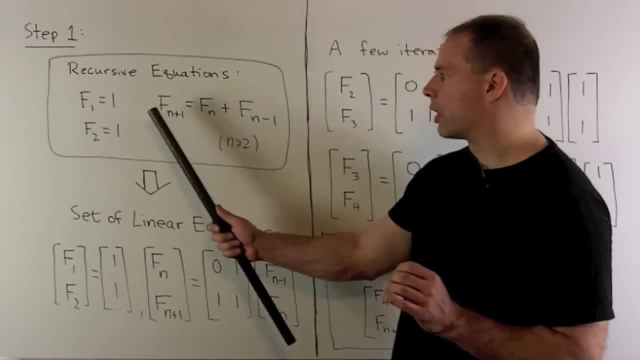 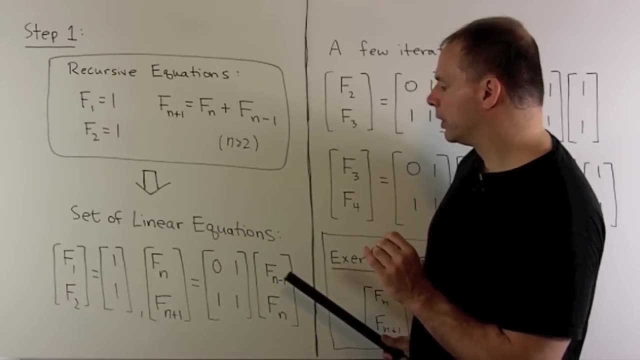 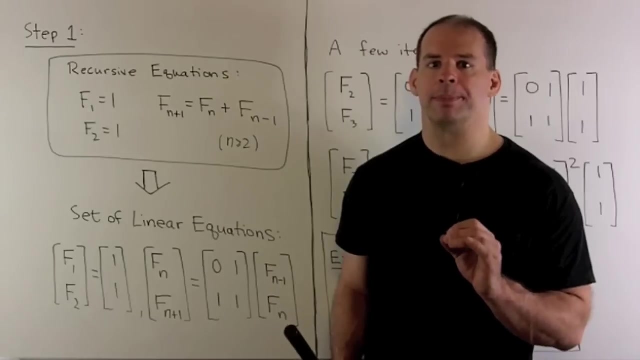 So I'm going to represent that as the vector For our recursive relation. we use this matrix vector product here. So if you multiply through the first row times, our vector just gives me f sub n. So we have the equation: f sub n equals f sub n. 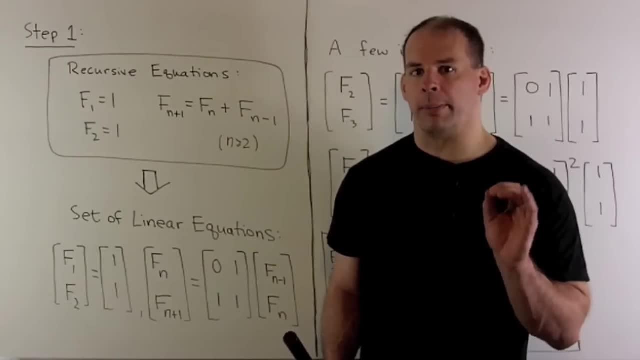 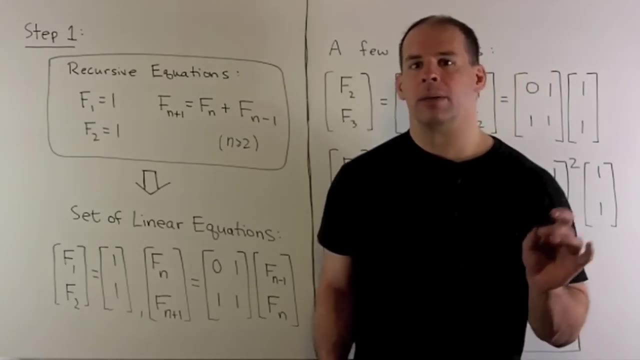 There's no content there, but I'll need that equation if I want a square matrix. Then if we take the second row times our column, we get f sub n minus 1 plus f sub n. That's equal to f sub n plus 1.. 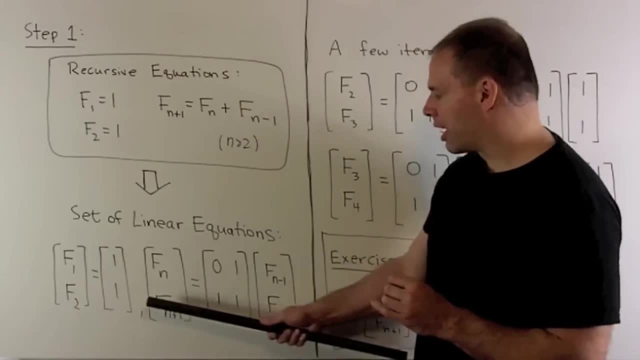 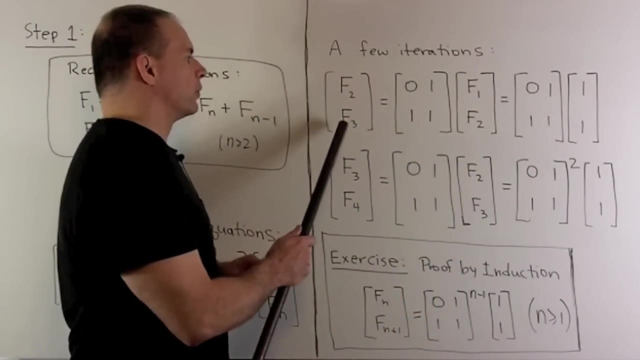 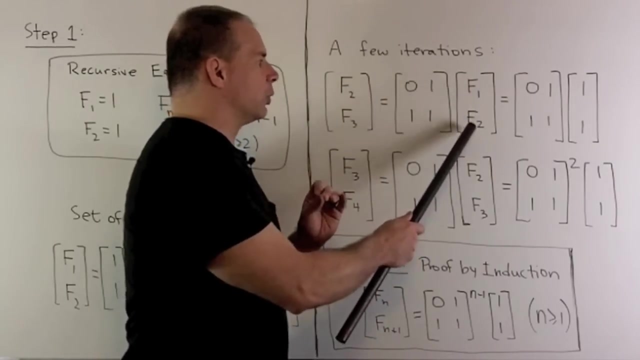 Now let's work out a few iterations of our matrix vector product here. So if I take f sub 2, f sub 3, we're going to take our matrix times, f sub 1, f sub 2.. So these are both going to be equal to 1.. 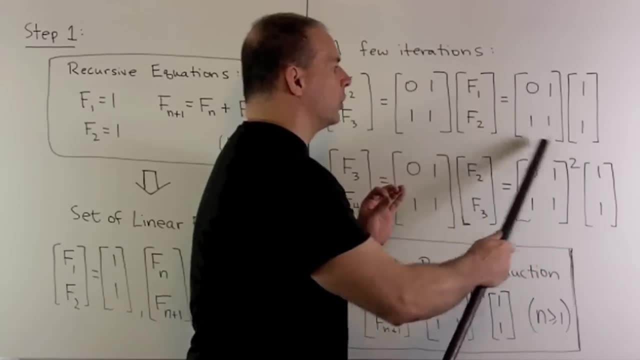 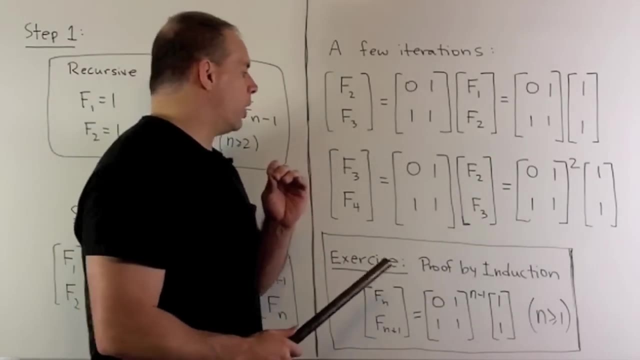 And then we get this product here. Now, we could work that out, but the idea is, I want to take a look at what's happening in the bigger picture. We do one more step. So if I want f sub 3,, f sub 4,. 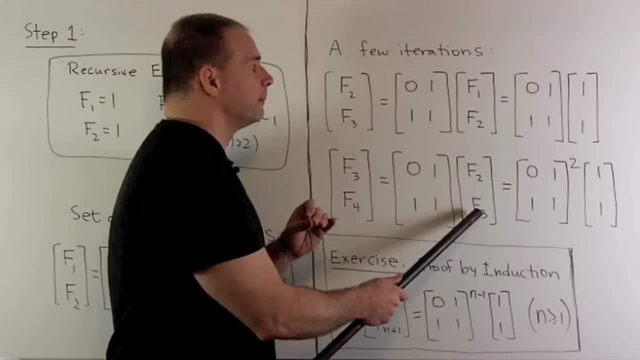 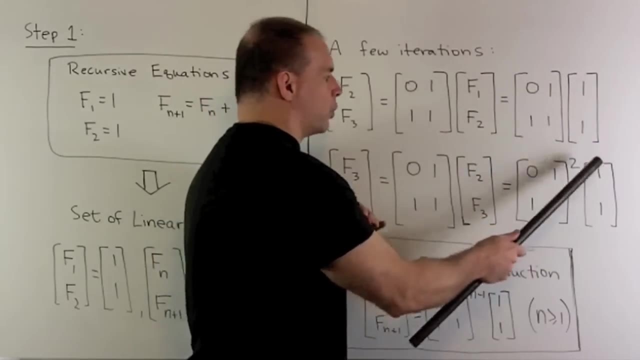 we take our matrix, multiply it by f sub 2, f sub 3.. Okay, then you note f sub 2, f sub 3. is this product right here? So we have our matrix squared times. Now, if you note what's happening, 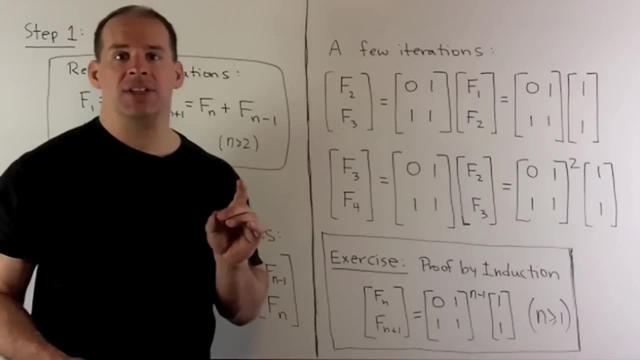 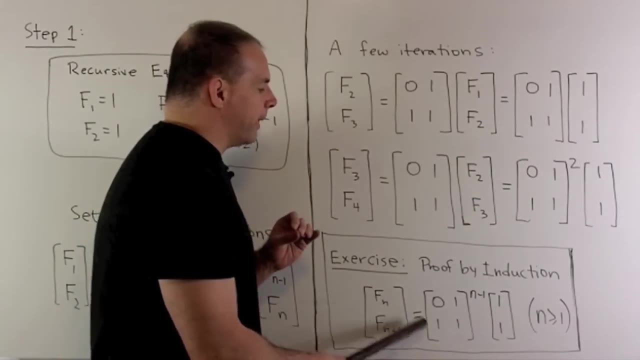 here's going to be a general formula, so I'll leave that as an exercise. So you should prove by induction that if I want f sub n, f sub n plus 1, it's going to be equal to our matrix, to the n minus 1 power times the vector. 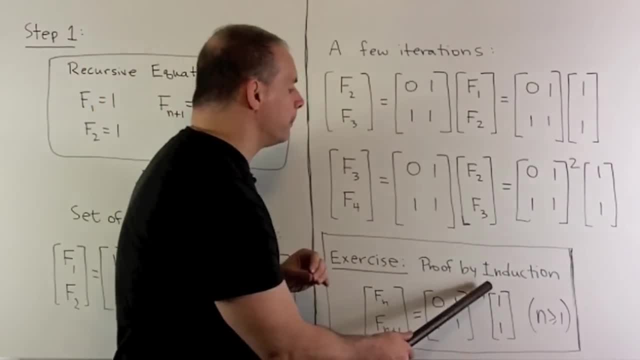 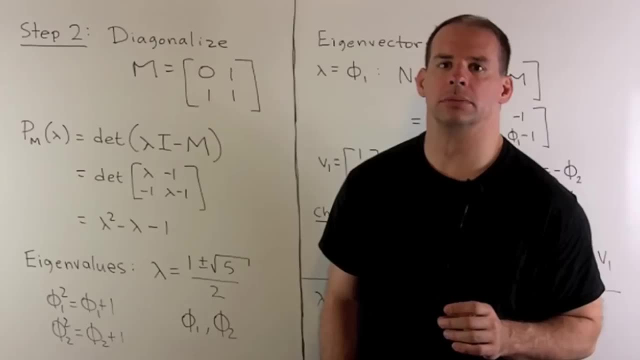 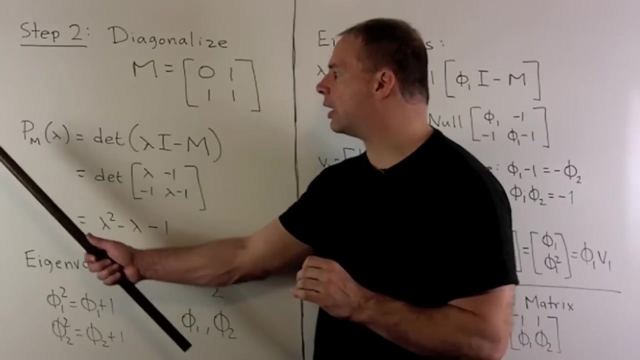 So now you note, we have a power of a matrix here. So if I can diagonalize this matrix, we have a chance of getting a nice formula out. Step 2, let's diagonalize our matrix. We start by computing the characteristic polynomial. 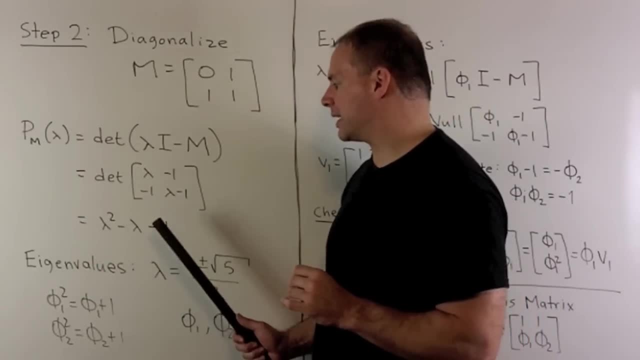 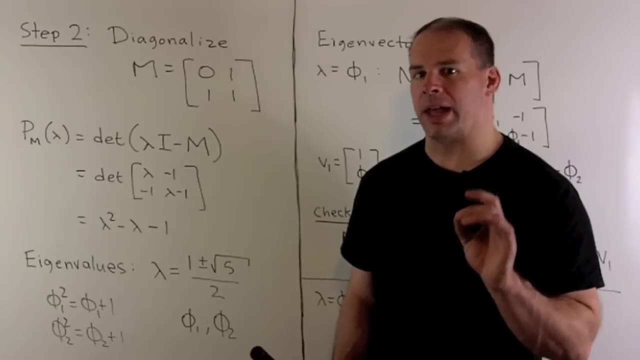 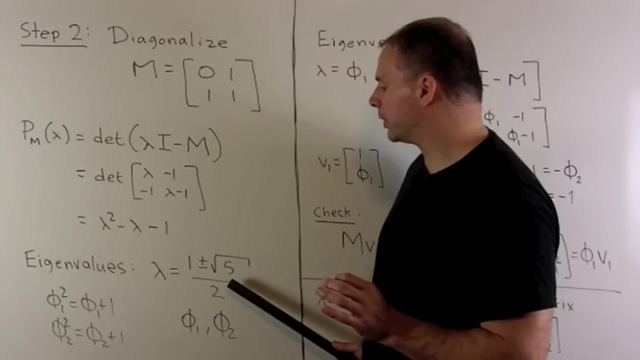 That gives us lambda squared minus lambda minus 1.. The eigenvalues are going to be the zeros of this polynomial. So I apply the quadratic equation. We get lambda equals 1 plus or minus square root of 5 over 2.. So we see where phi 1 and phi 2 come into the picture. 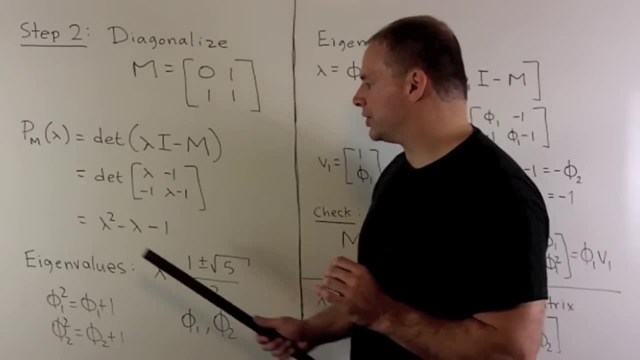 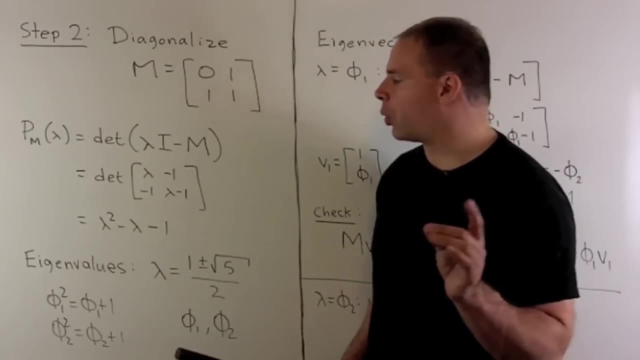 Now, because phi 1 and phi 2, because phi 1 is 0. for this polynomial we're going to have: phi 1 squared minus phi. 1 minus 1 equals 0, or phi 1 squared equals phi 1 plus 1.. 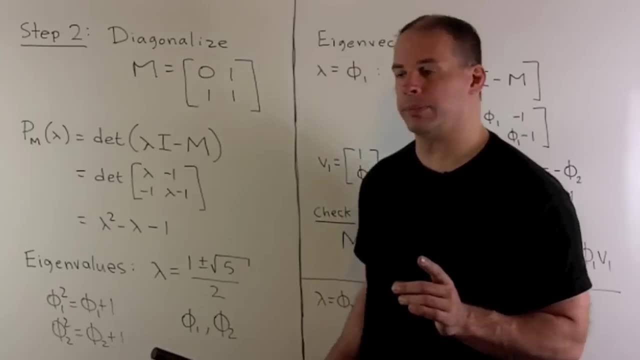 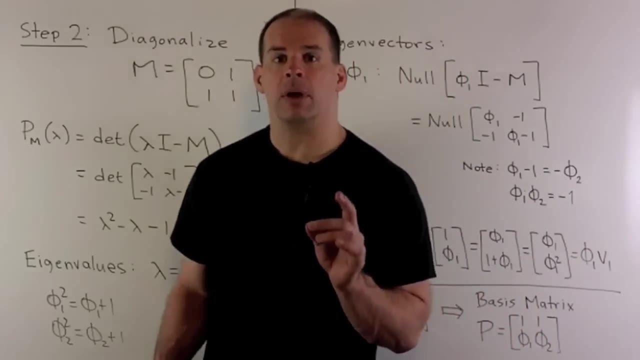 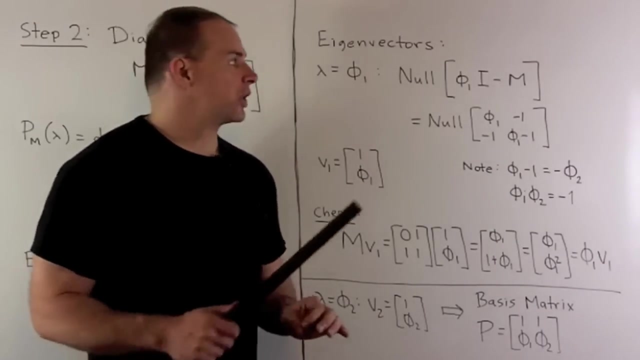 Okay, so we can work that out directly if we wanted. We also have similar formula for phi 2.. Now with our eigenvalues, we want to find eigenvectors for each eigenvalue, So for lambda equal to phi 1,. 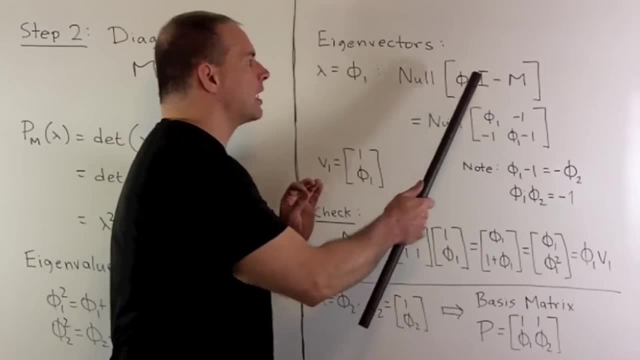 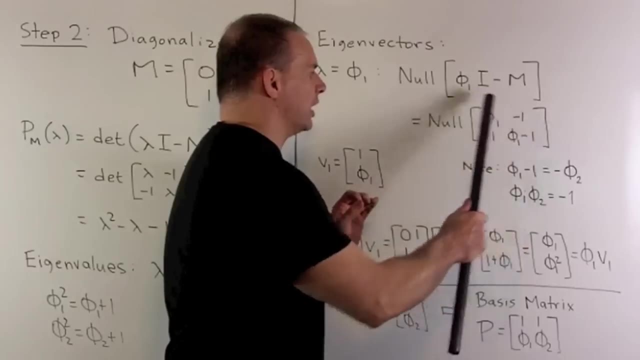 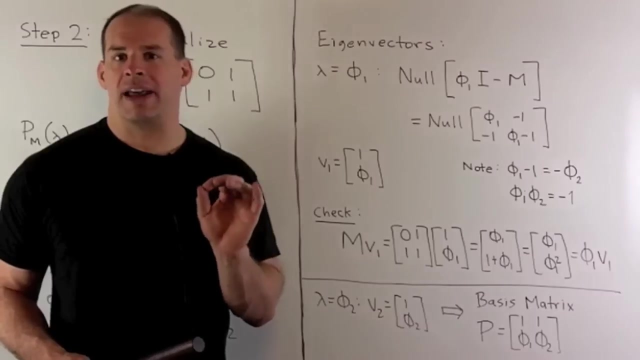 we're trying to solve for the null space of phi, 1 times i minus our matrix. We're trying to find the null space of this matrix here. Note that the null space is going to be more than just 0. So all I need to do is to find a vector that zeroes out the first row. 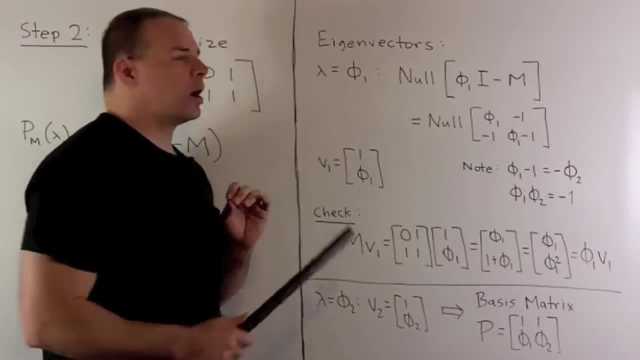 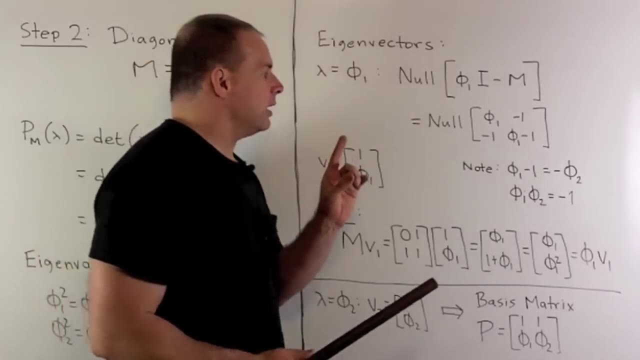 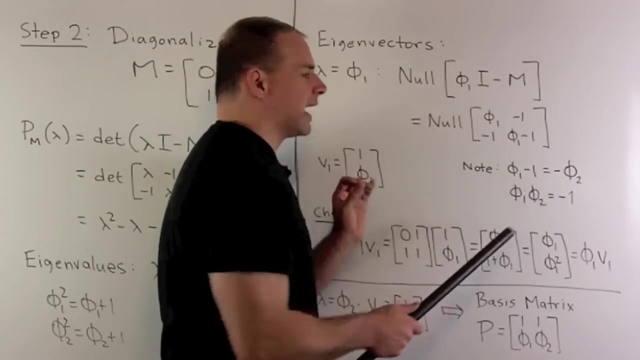 Okay, the vector that will do that is going to be v1 equal to 1 phi 1.. Now, if you wanted to row reduce, then you're going to need the identities: phi 1 minus 1 equals minus phi 2, and phi 1 times phi 2 equals minus 1.. 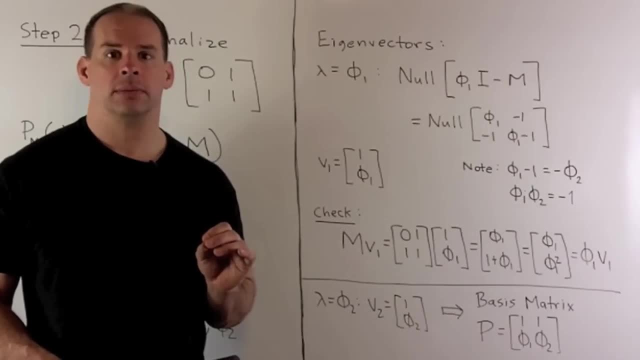 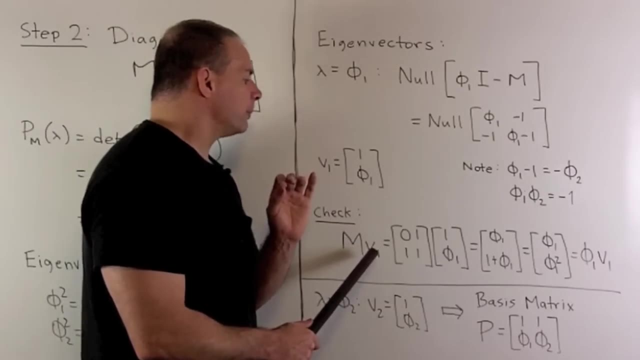 And then you can get your answer that way. Now we check our work, of course. So we take our matrix, multiply it by our eigenvector. You'll note when we take the product, we get phi 1, 1 plus phi 1.. 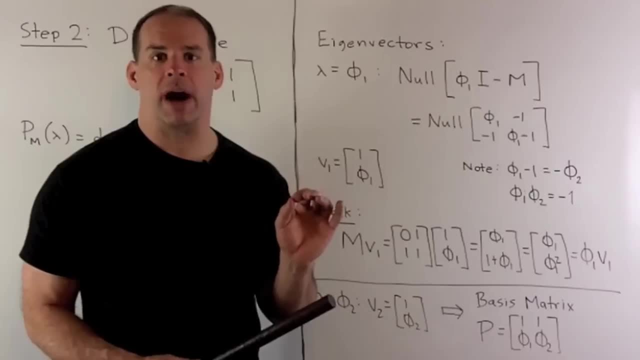 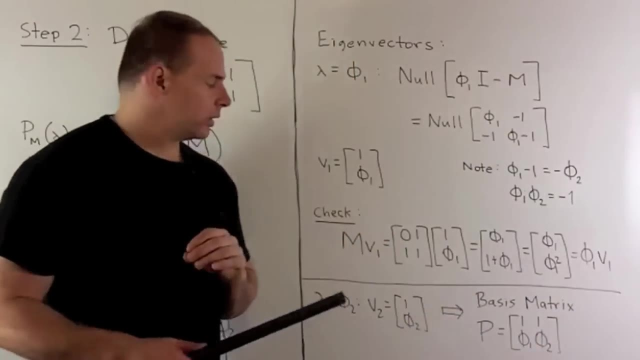 But we've already seen that 1 plus phi 1 is phi 1 squared. So I factor out a phi 1, and that gives me phi 1 times v1.. That checks our work. So our matrix times v1 gives me phi 1 v1 back. 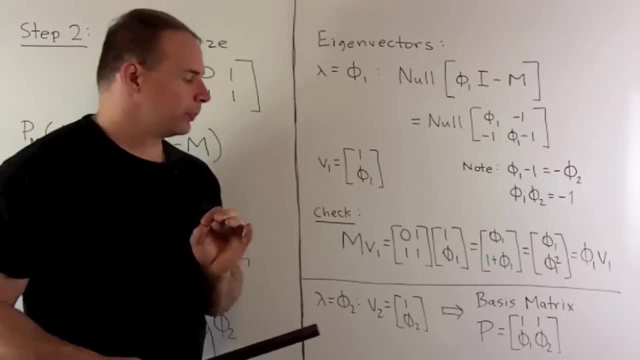 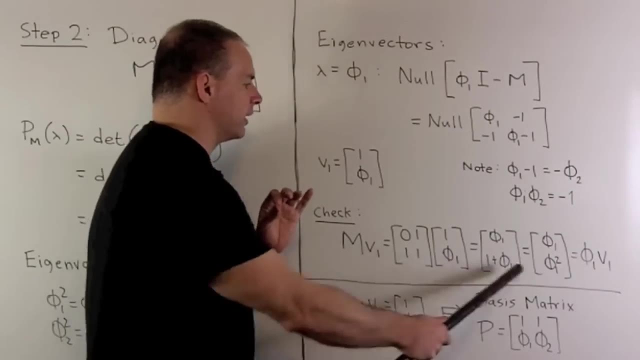 Now you could do all that same work for phi 2.. Then our eigenvector is going to be 1, phi 2.. We'll call that v2.. Okay, you could check everything here. That gives us a basis of eigenvectors. 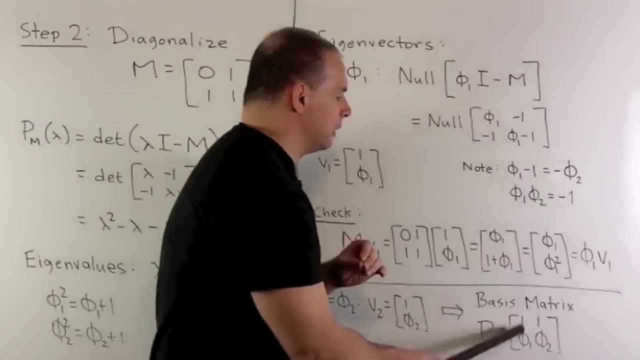 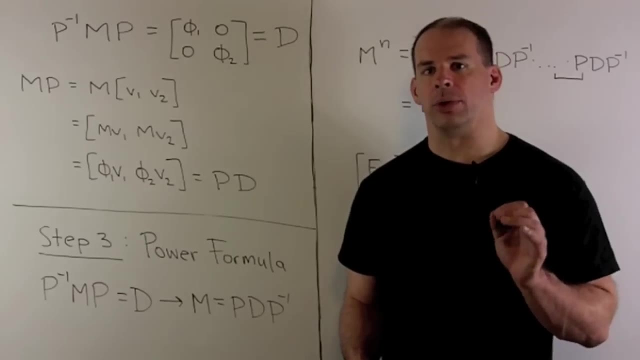 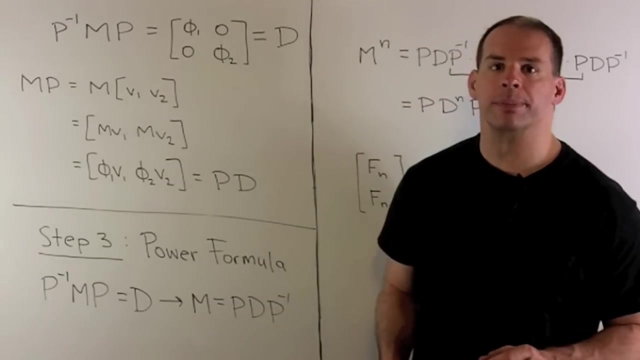 So we set up our basis matrix P as v1, v2 or 1, 1, phi, 1, phi 2.. How do we use our basis matrix? The formula is: P inverse MP is equal to our diagonal matrix, where the diagonal entries are our eigenvalues. 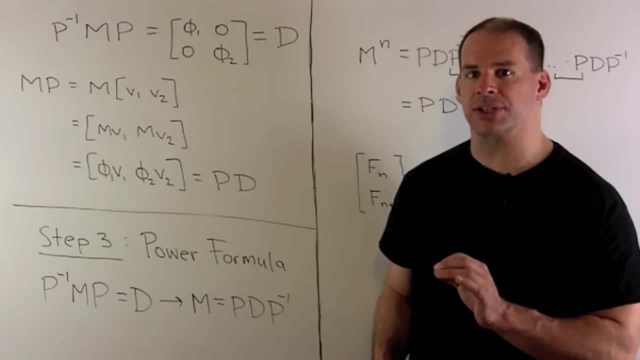 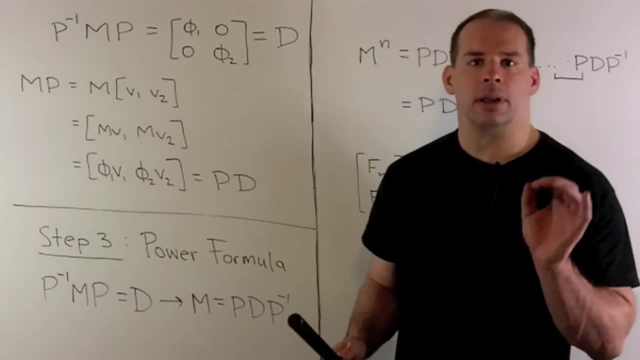 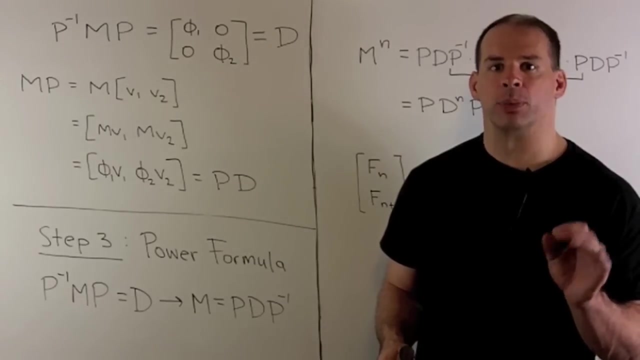 in the same order that we've ordered our eigenvectors in the basis. Now to see this: if I multiply M times P, then we're just multiplying M by each column vector. Since the column vectors are eigenvectors, we just multiply by the corresponding eigenvalue. 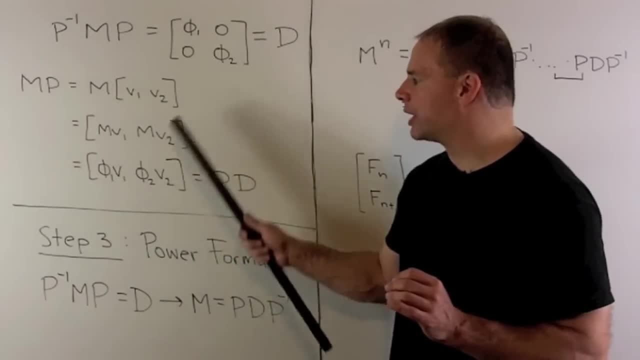 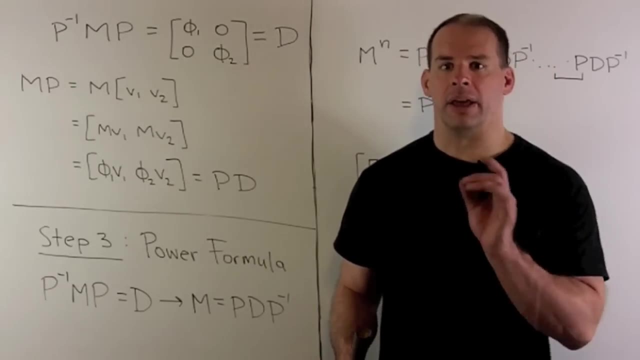 And then if I want to multiply the columns by scalars, that's going to be by multiplying by a diagonal matrix on the right-hand side. If we multiply by a diagonal matrix on the left-hand side, that's going to push the scalars into the rows. 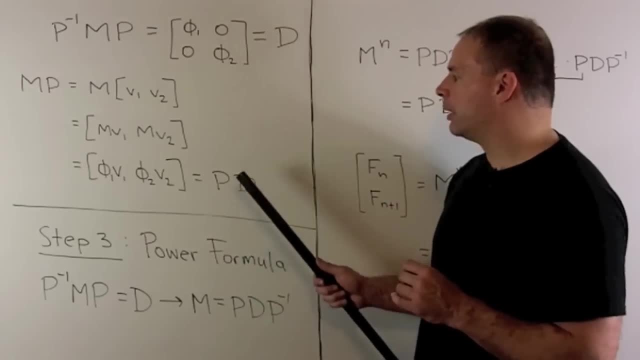 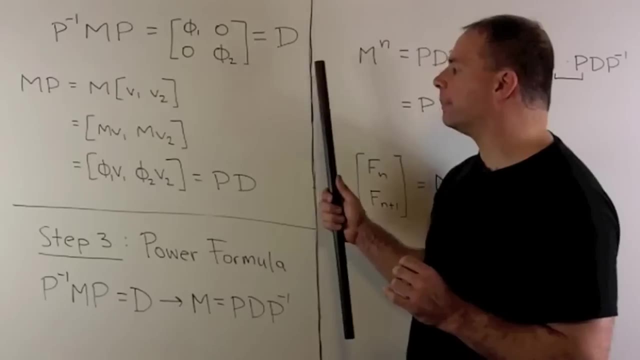 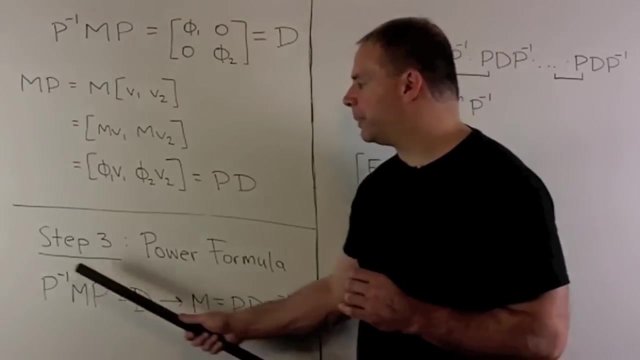 Then we just push P to the other side as P inverse. Now to apply this formula here, I'm going to use the power formula for a matrix. First I want to isolate M, So I push the P inverse and the P to the other side. 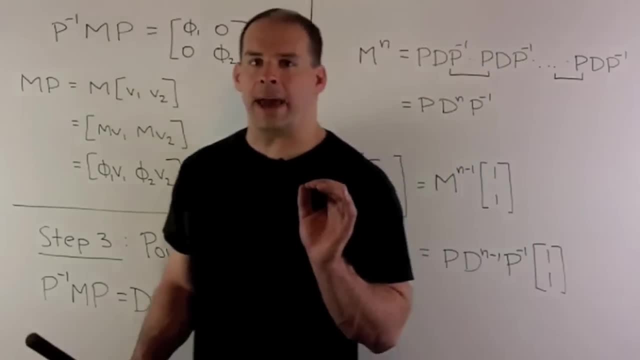 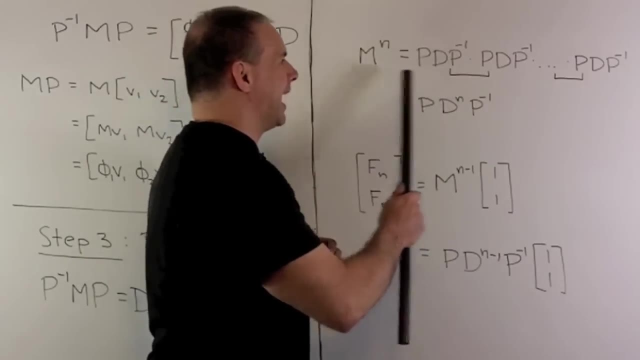 If I take M to a power? what happens? So if we take M to the N? well, I'm going to write P, D, P inverse out N times And then you'll note the P inverse P's are going to cancel out. 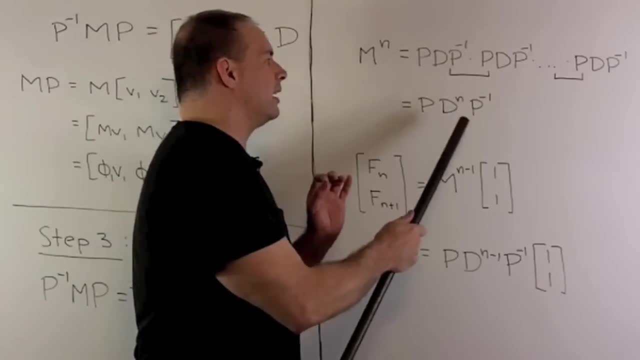 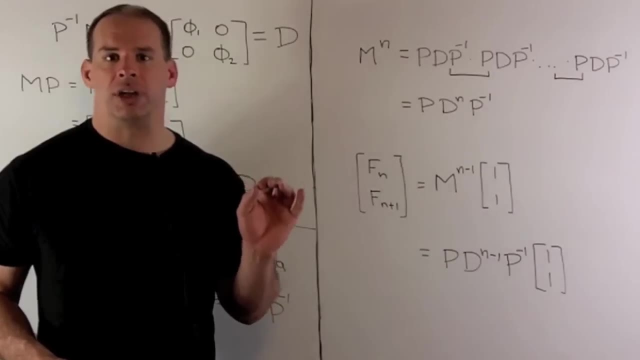 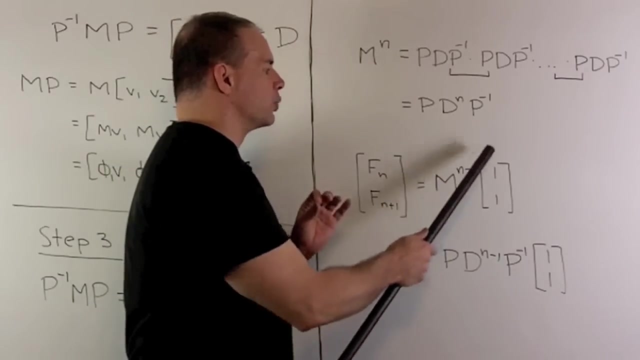 and this collapses to P D, to the N P inverse. If we go back to our matrix vector formula for the Fibonacci numbers, we have F sub N. F sub N plus 1 is equal to M, to the N minus 1 times 1, 1.. 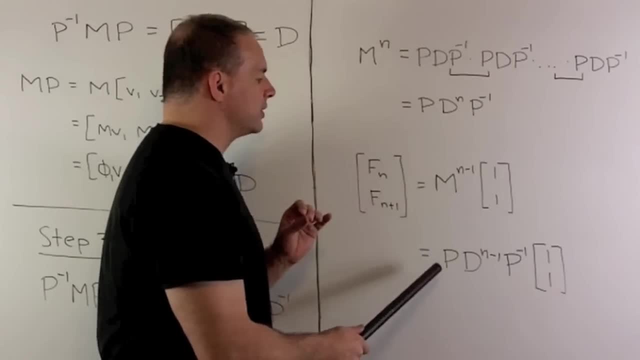 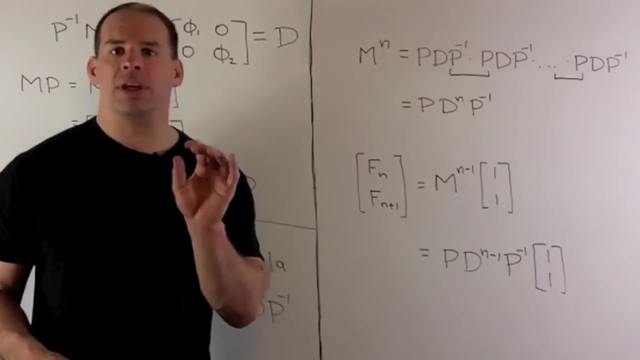 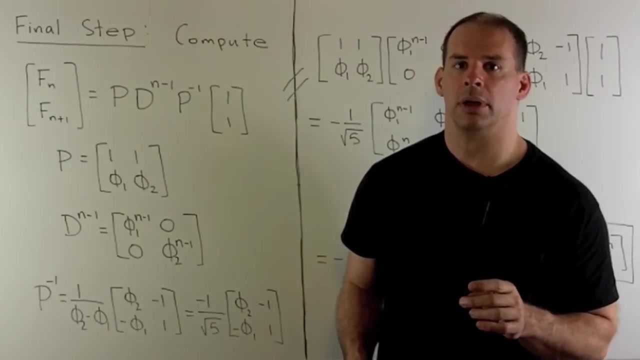 We sub in for our M, What we'll have is P D to the N, minus 1 P inverse on our vector 1: 1.. So now we can start pulling the numbers out of this Final step. we compute, We start with our final formula. 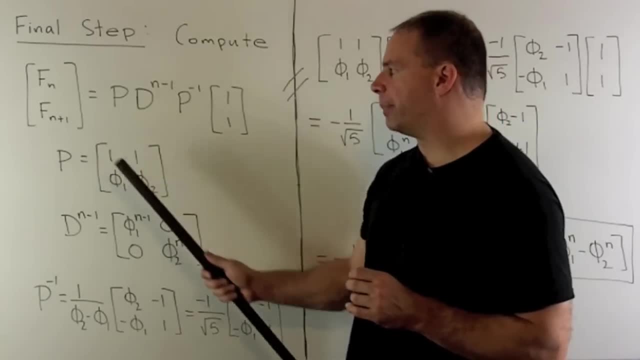 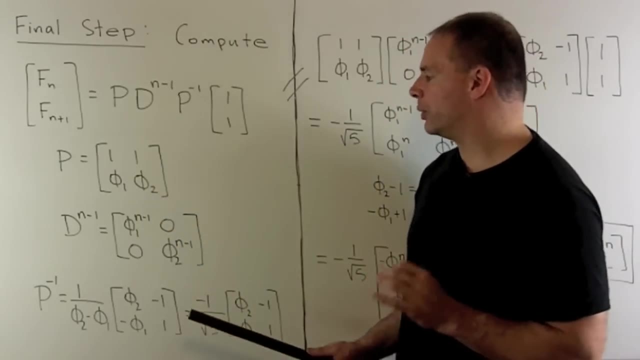 Where are the items we have here? P is our basis matrix 1, 1 phi 1, phi 2.. D to the N minus 1 is just a diagonal matrix with diagonal entries: Phi 1 to the N minus 1, phi 2 to the N minus 1.. 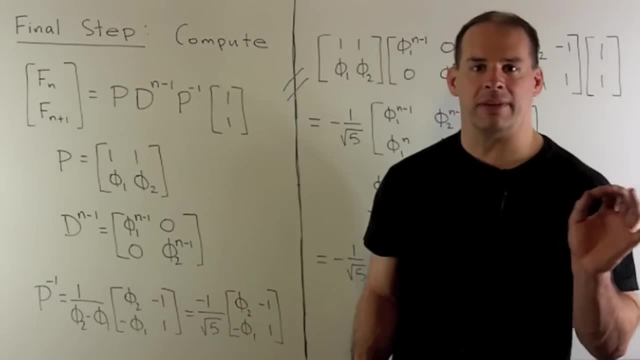 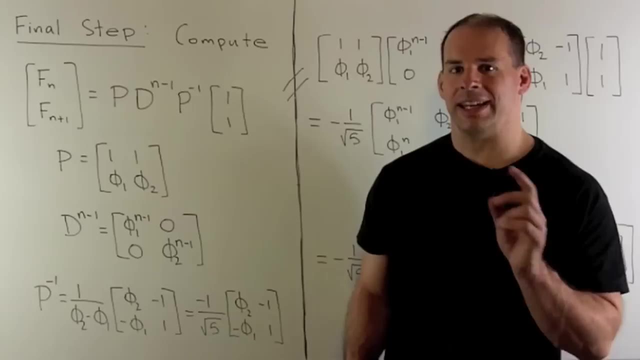 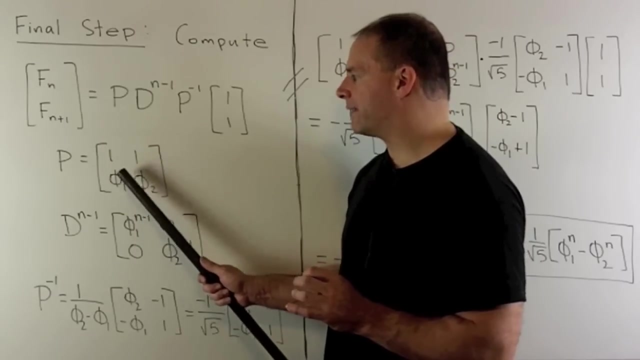 Then for P inverse, we just use our rule for computing the inverse of a 2 by 2 matrix, So it's going to be 1 over the determinant. I switch the entries on the diagonal and negate the entries off the diagonal, So I'll have phi 2 and 1 minus 1 minus phi 1.. 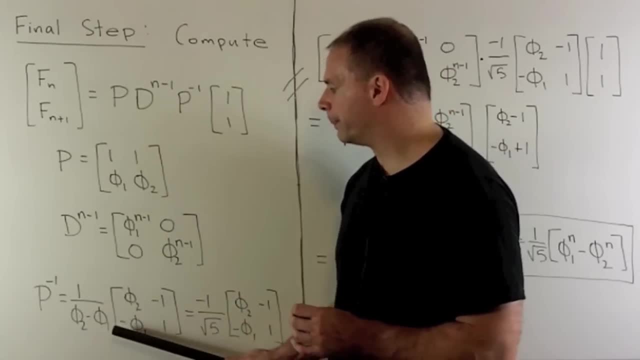 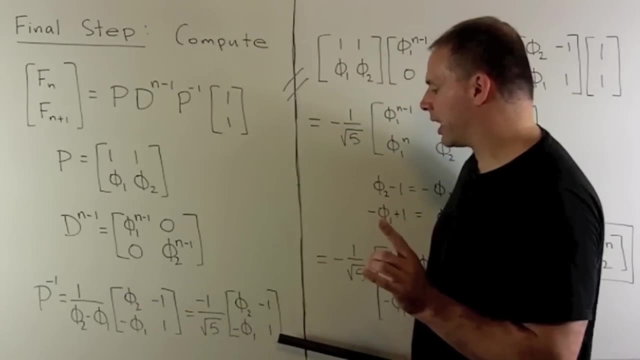 Our determinant is just going to be phi 2 minus phi 1.. Now the determinant is going to collapse to 1.. It's going to collapse to minus square root of 5.. So we'll just keep this like this for now.